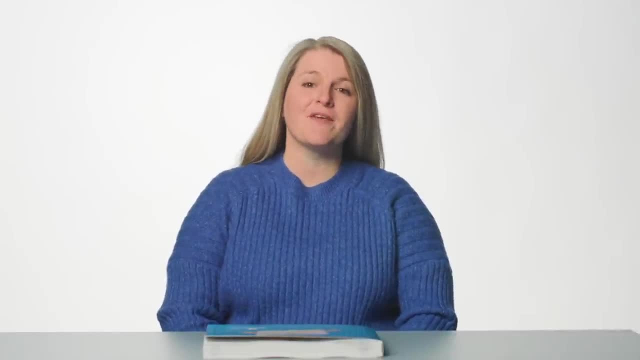 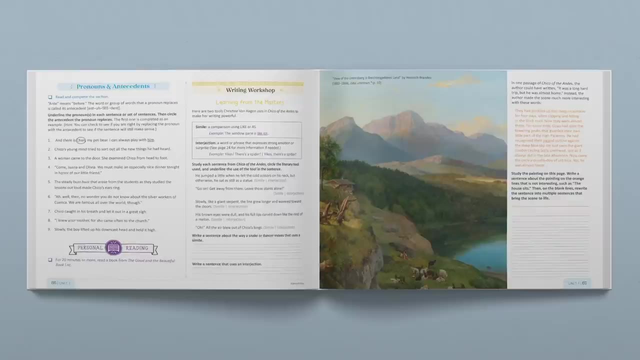 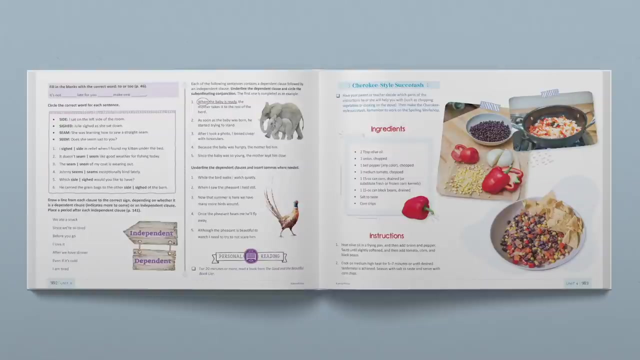 Hi, it's Jenny Phillips. I'm excited to do a flip-through of the Level 5 Language Arts course for The Good and the Beautiful. Each lesson is carefully designed to be academically strong, maximize learning time by connecting multiple subjects, create strong spellers and writers and explore the beauty and the power of art, geography and literature. 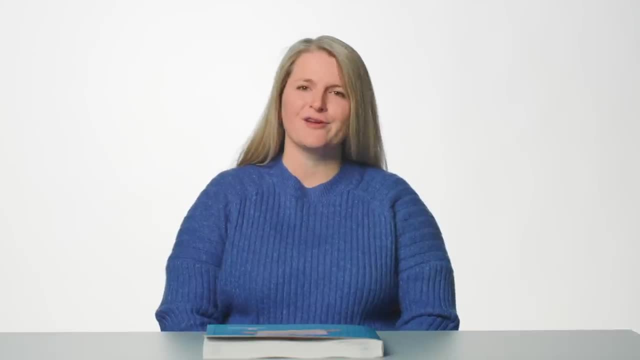 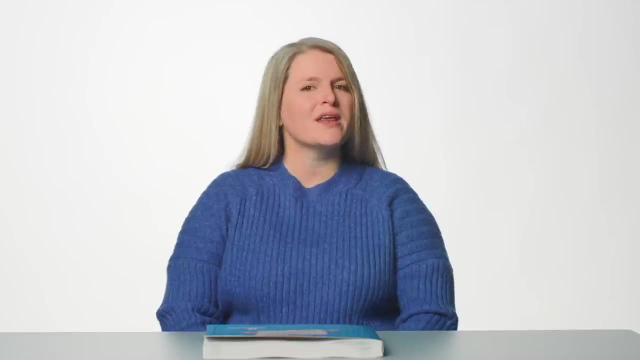 The entire course is available as a free download on goodandbeautifulcom. And, like all of our Language Arts courses, the following subjects are integrated into one course: Reading, writing, literature, spelling, geography, art appreciation, art instruction, grammar usage and punctuation. 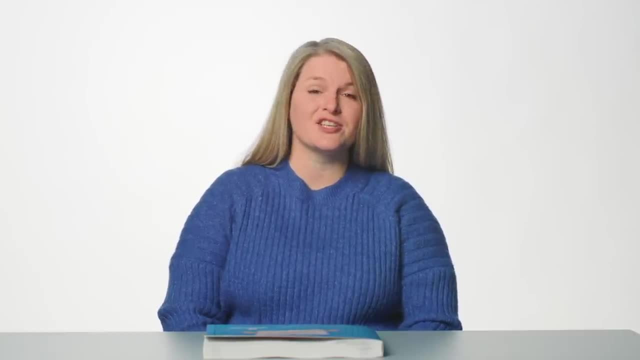 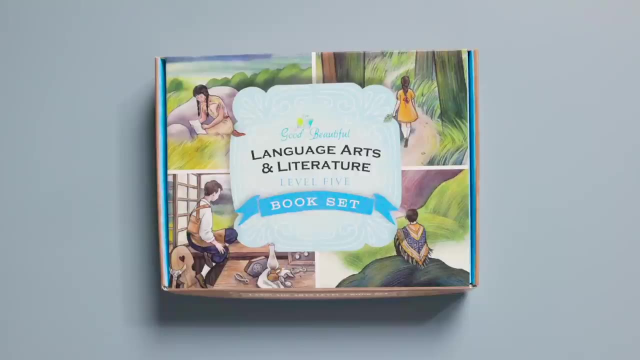 and even a little bit of baking and cooking that's connected to the literature in the course. The Level 5 course set comes with three items: The Level 5 course book, the Level 5 book set and the geography and grammar cards. 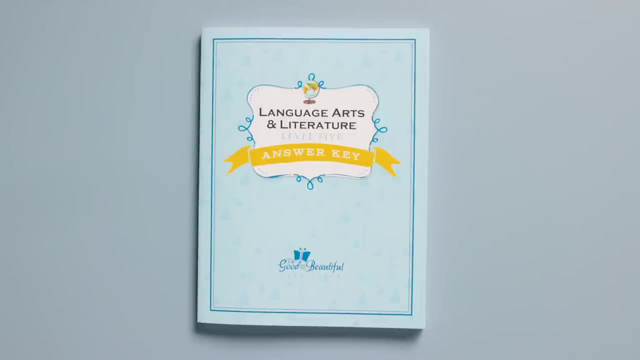 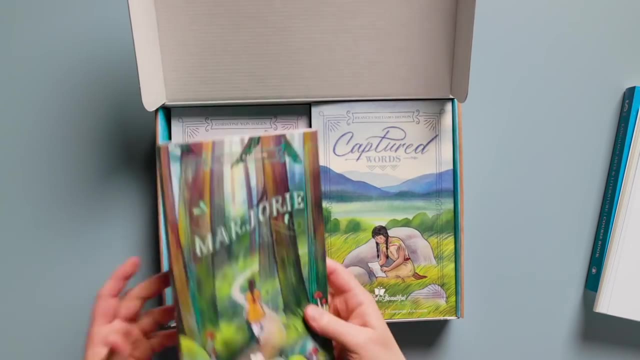 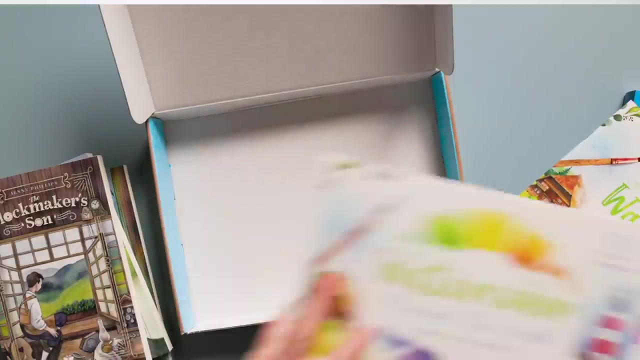 An answer key is also available. The Level 5 book set is also available as a download, or a physical answer key is available to purchase. The Level 5 book set comes in a sturdy box so you can keep the items stored together. In the box are four full-length books, a watercolor instruction book and a watercolor pad with templates that come shrink-wrapped together. 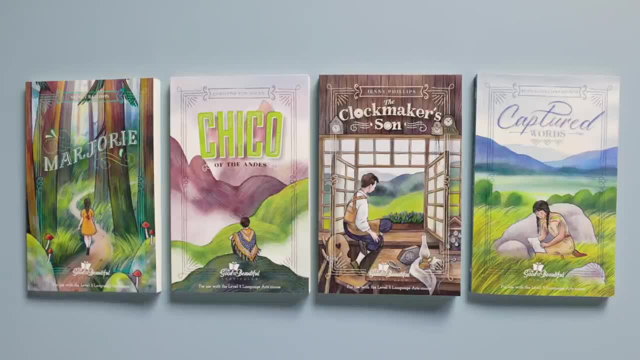 Let's take a look at the books that are integrated with the course. They are all packed with high moral, educational and literary value, And we also made sure our pilot children love them. First is Chico of the Andes, written in 1910.. This book was published in 1843.. This book takes place high in the Andes Mountains of Ecuador. Next is Marjorie, written in 1950.. The book is set on an island off of the coast of Maine. Then we have The Clockmaker's Son. 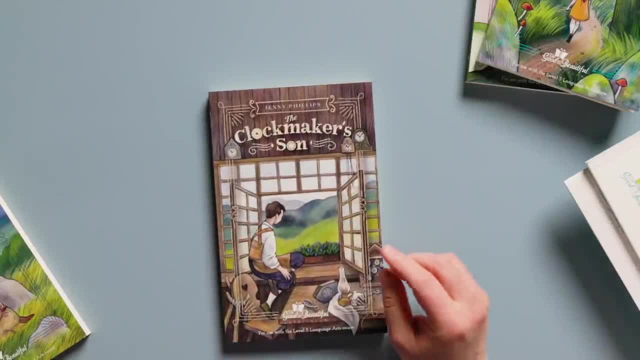 Some of our editors said that this book made them laugh and cry and even changed them for the better. And last we have Captured Words, a biography that tells the incredible story of Sequoia, who, against all odds, worked to create a written form of the Cherokee language with the help of his daughter. 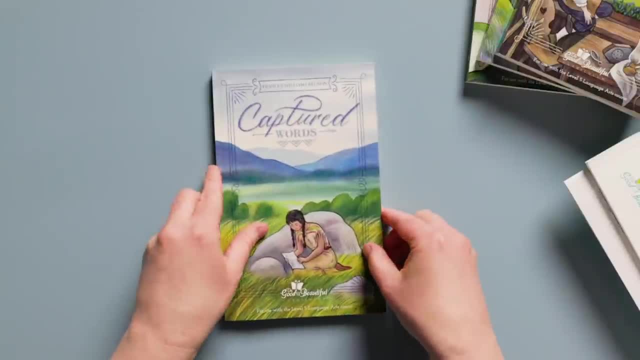 In this book we also have the author of The Clockmaker's Son. This book is written in 1910.. The author of The Clockmaker's Son is the author of The Clockmaker's Son. The author of The Clockmaker's Son is the author of The Clockmaker's Son. 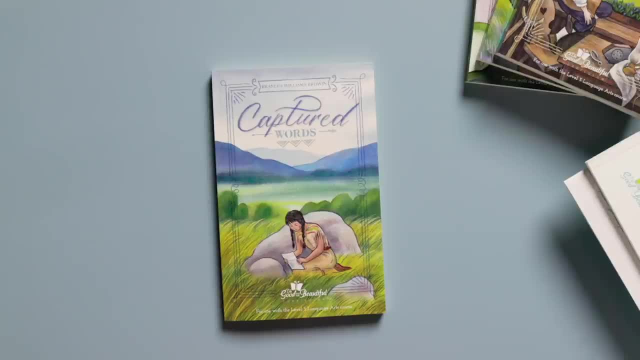 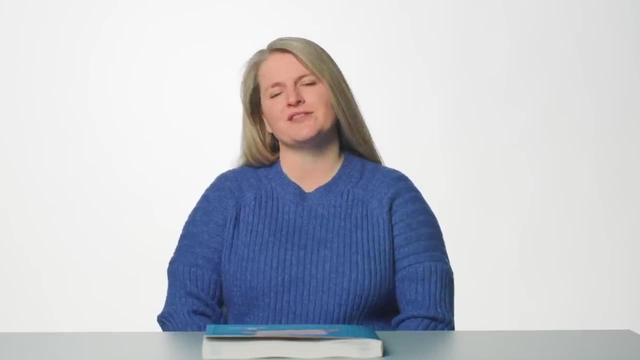 The author of The Clockmaker's Son is the author of The Clockmaker's Son. In addition to these books, lessons in the course direct the child to listen to a classical book titled Gabriel and the Hour Book by Evelyn Stein, which is set in the Middle Ages. 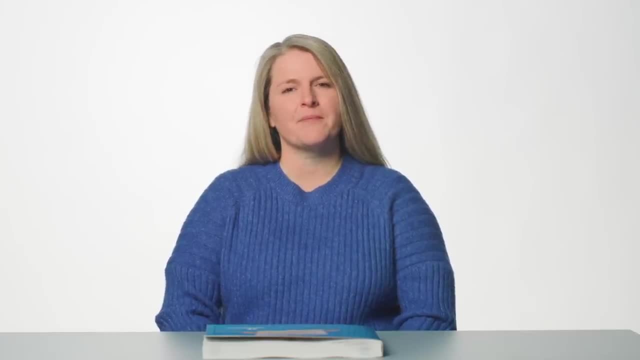 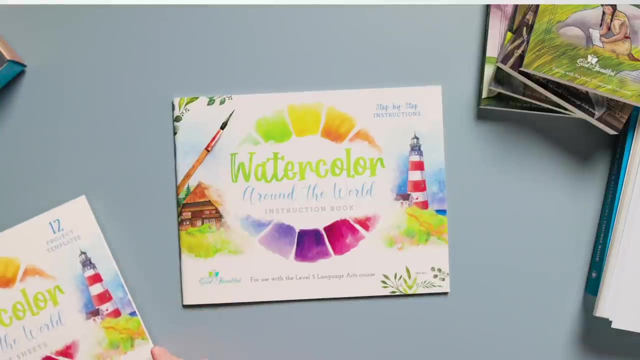 The audiobook is available on our free homeschooling app. For each of these books, the course book tells you when to read the books and how to use them. The next component was a big favorite with our pilot families. The watercolor book has step-by-step instructions for 12 projects that are integrated throughout the course. 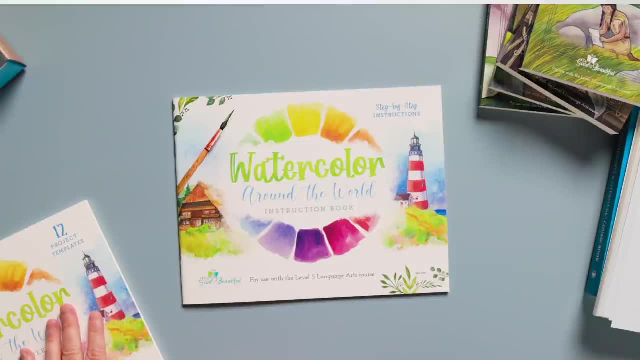 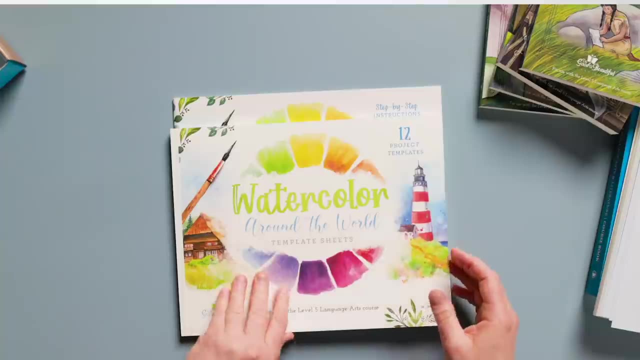 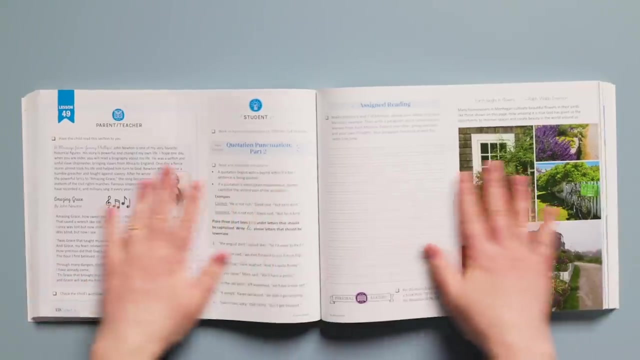 Each project is connected to what the students need. Each project is connected to what the students need. Each project is connected to what the students need, And the book comes with an accompanying watercolor pad with light gray templates on high-quality watercolor paper to make the projects easier and more fun for the child. 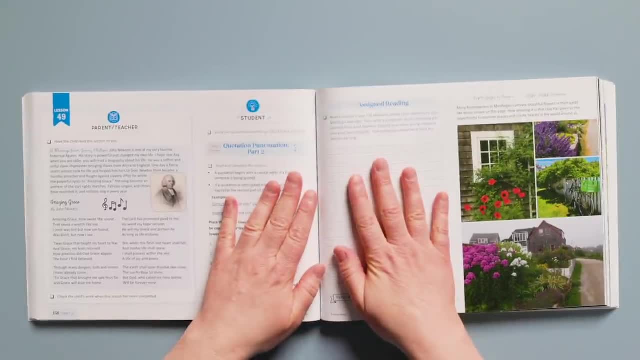 So now let's take a look at the course book. The 398-page book does not have bulky coil binding. Rather, the book is bound with lay flat, perfect binding, which allows the child to work on pages without the books starting to close. 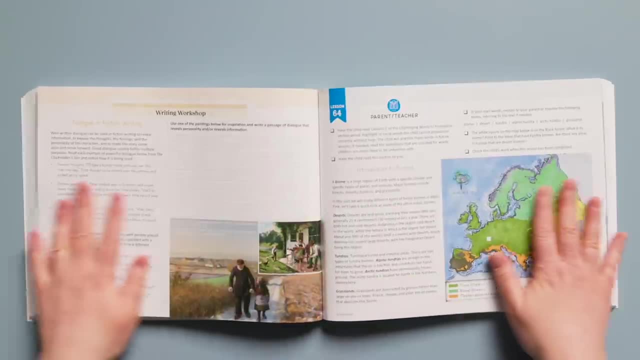 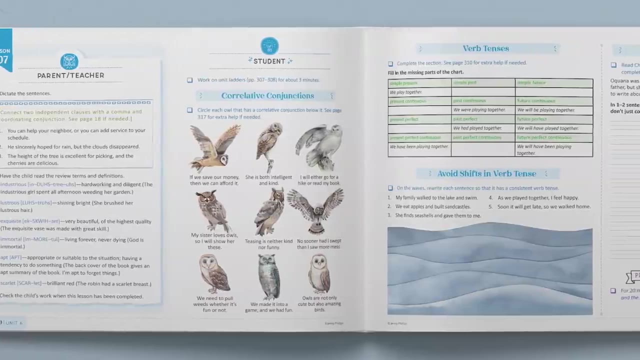 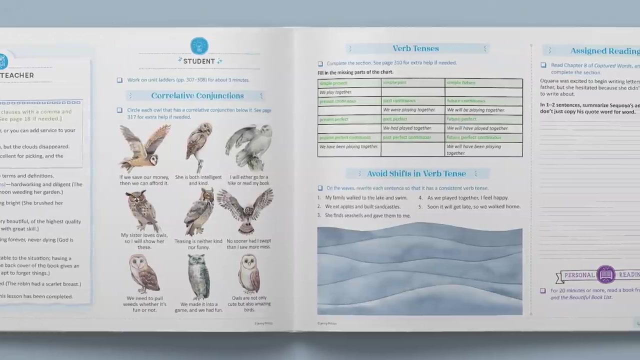 you want to take them out. We recommend keeping a sticky note on the current lesson. The course is mainly student-directed, but each lesson starts with a short section that the parent completes with the child. The child then completes the independent sections of the lesson. Every lesson ends with either a writing workshop or a spelling workshop. 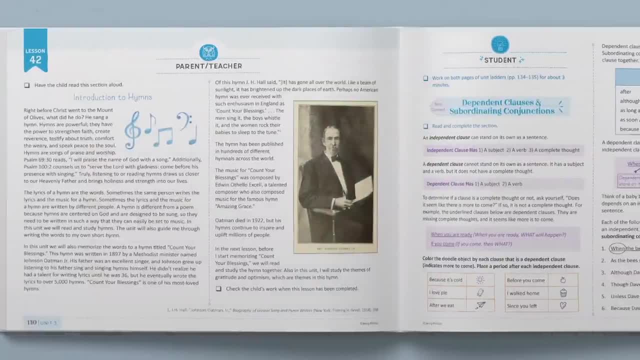 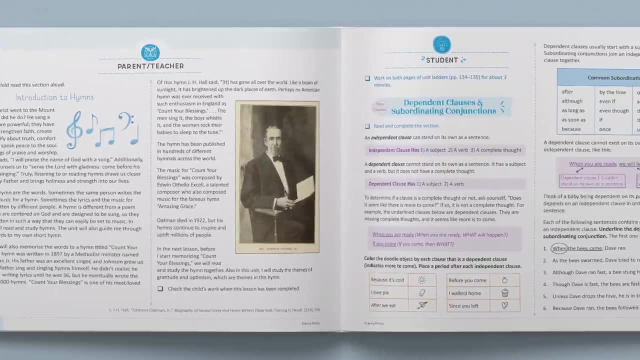 found right in the course book For the parent-teacher section of Lesson 42, the child reads An Introduction to Hymns to the Parent. This allows the child to read advanced text, with the parent guiding the child through any difficult words. The child also gains knowledge about hymns and their 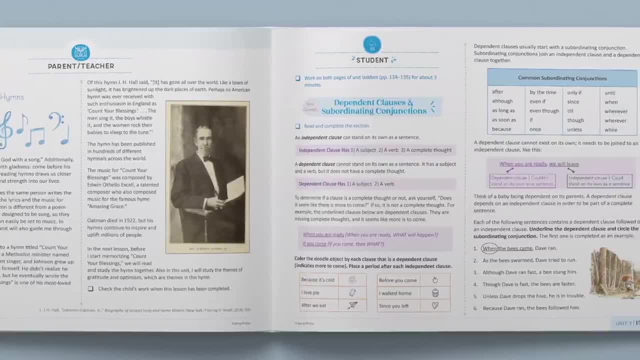 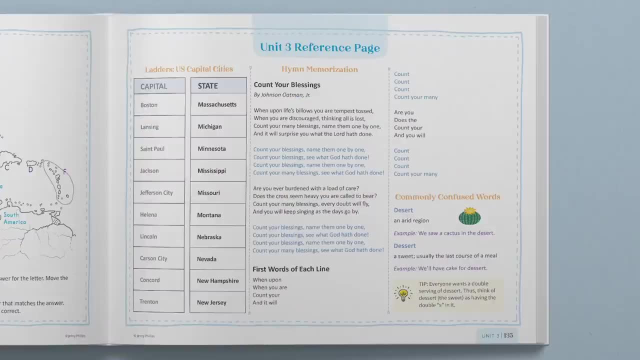 power and is inspired while reading the story behind the hymn Count Your Blessings. The course guides the child through memorizing this hymn, which contains powerful words that will always remain with the child. The child then completes the student section for Lesson. 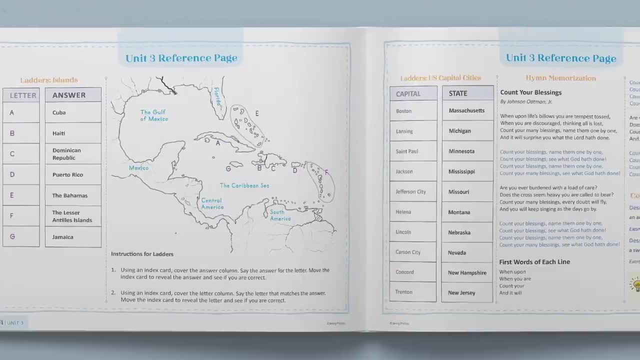 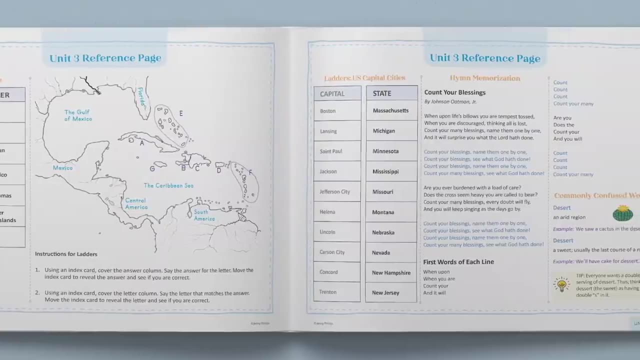 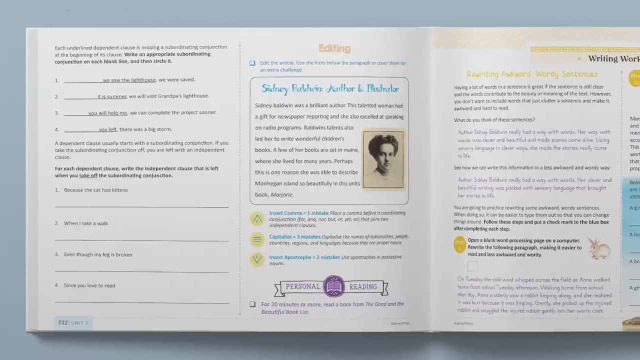 42, which first directs the child to work on memorizing US state capitals. The child will also memorize Canadian provinces and territories, the location and names of the islands and more in this course. Next in the lesson, the child completes a grammar section, then completes an editing. 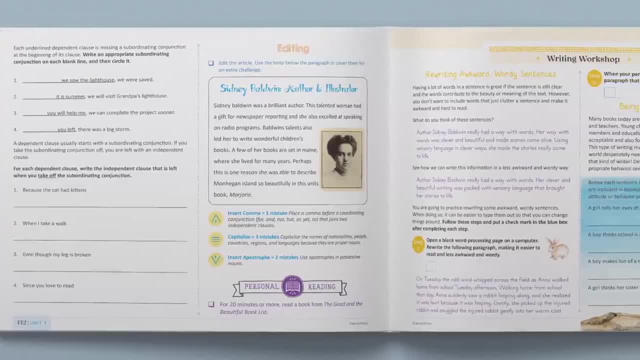 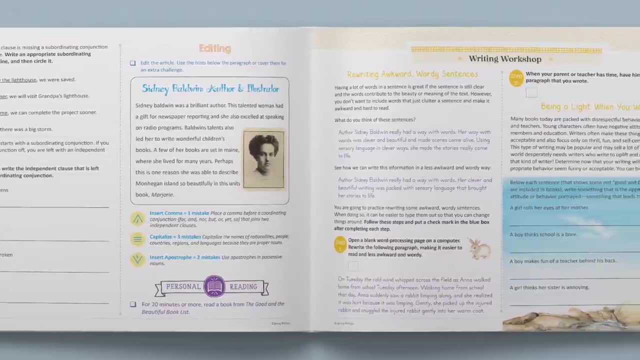 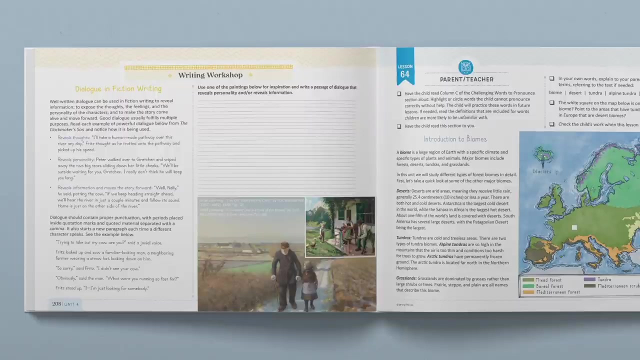 section which also doubles as a biography of Sidney Baldwin, the author of the book the child is about to read. Finally, the child completes a writing workshop. These writing workshops are a highlight of our courses, as they create strong, beautiful writers. The writing workshops integrate art. 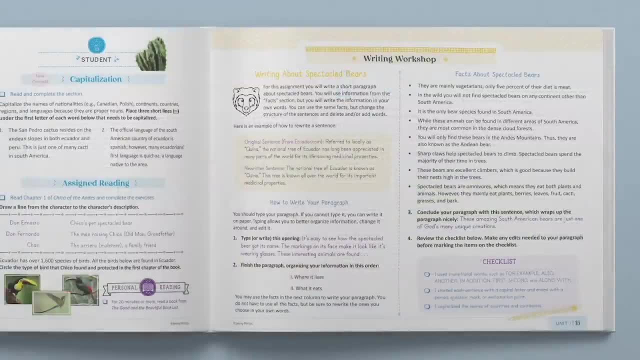 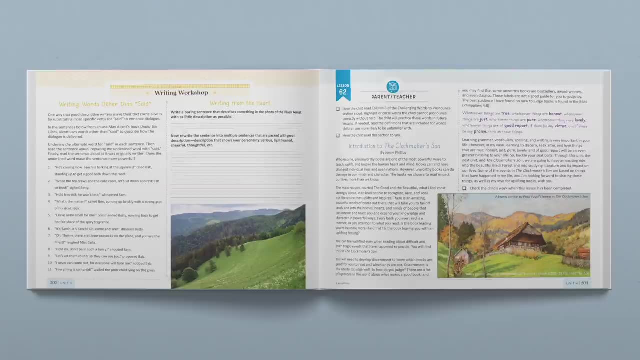 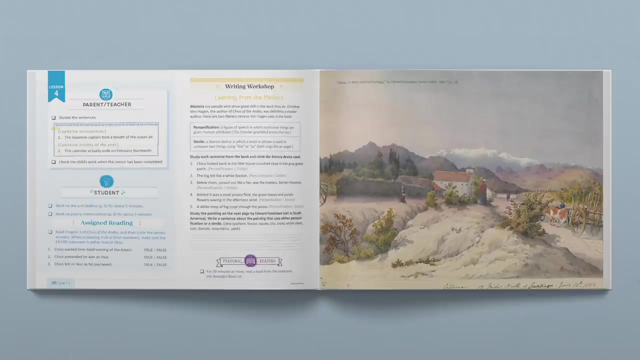 geography and literature that connect the child to the world. The child then completes the integrated books and the art and geography being studied. Some writing workshops focus on exercises to improve writing in specific ways and to encourage the child to write from the heart and enjoy writing. At times the child does writing workshops titled Learning. 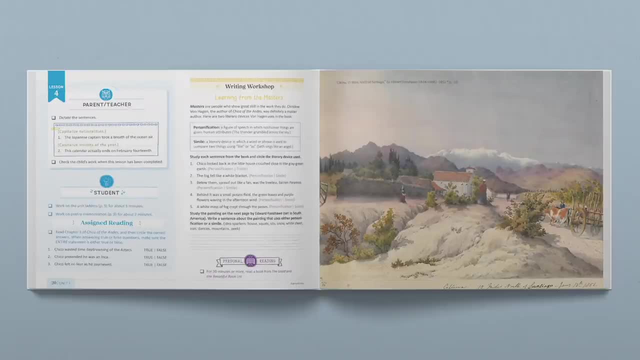 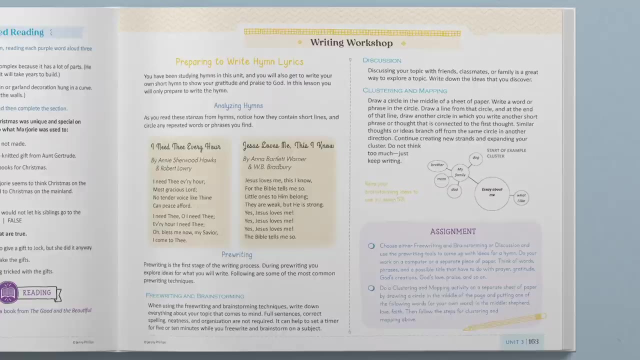 from the Masters, where the child studies and learns from the best authors. The writing workshops gently lead the child through many full-length writing projects, such as hymn writing, essay writing and more. The child then completes a grammar section. These writing workshops are a highlight of our courses as they create strong, beautiful, beautiful. 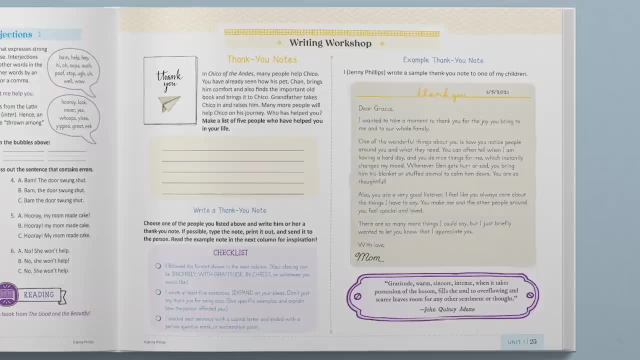 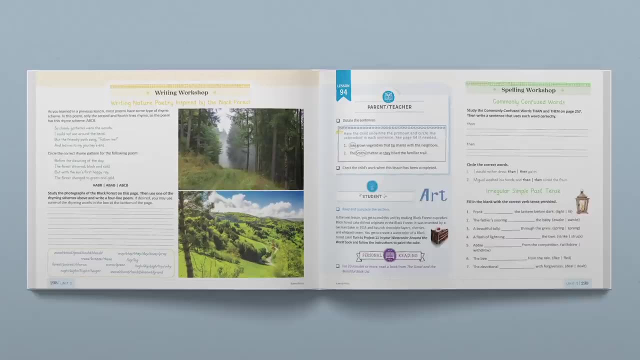 and effective writers. The child syllabus is Nay printing, internet writing. thank you, note writing, storytelling, geography articles, family newsletter, book review, nature, poetry and more. This, this, Don't be afraid to go from grammar to theater. 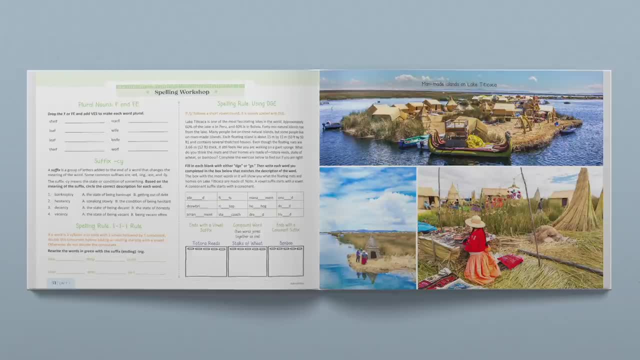 To forbid the child from considering other lattice先 Miloans and to avoid it from ourselves. regular reading and communication is essential. Put your relies on the teacher and help them. The spelling workshops which are included in every other lesson are a powerful and 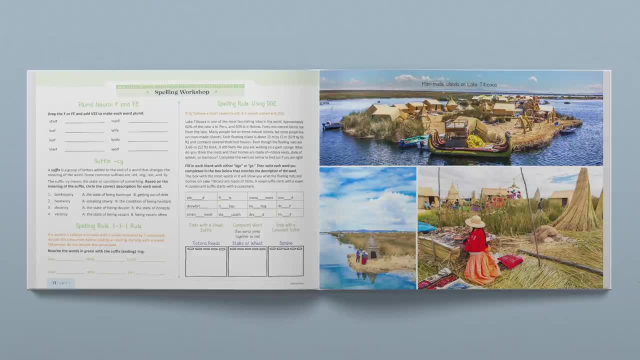 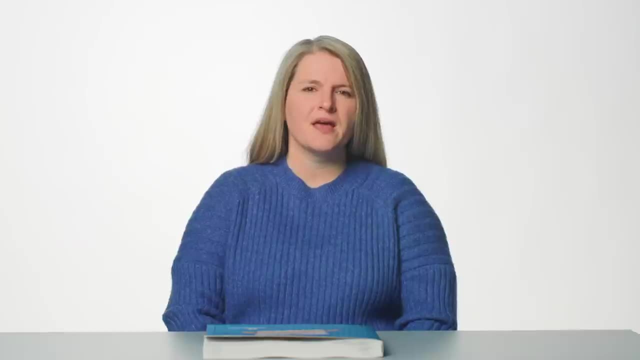 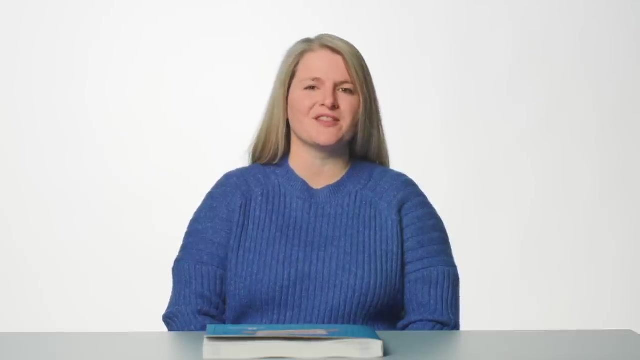 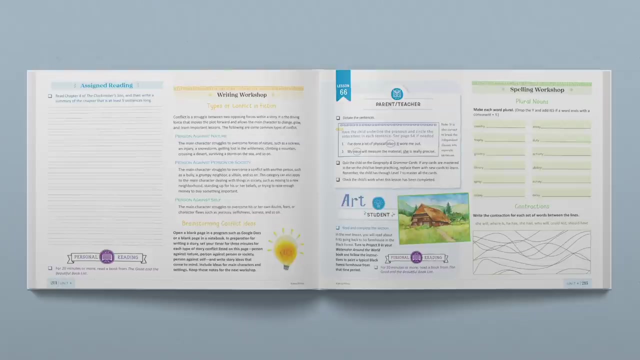 fun way to create strong spellers�. Sub intellectual studies, Introduction, preparatory voice, industries, 달 English- same every day, so the child does not get fatigued and is always excited to see what the lesson holds. In Lesson 66,, for example, the parent section covers spelling, dictation and reviewing geography. 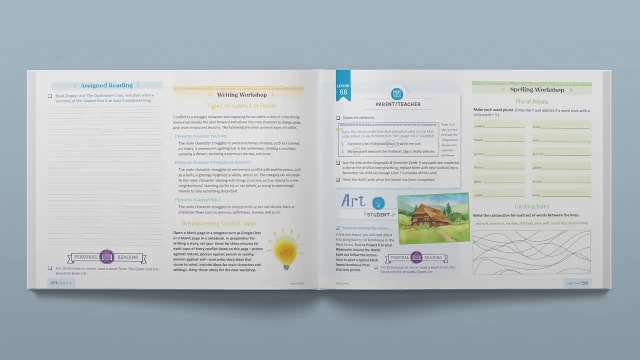 and grammar cards with the child. The student section instructs the child to complete an art project correlated with the Black Forest, which is a theme of the unit, and the child also completes a spelling workshop. In Lesson 92, the child reads nature poems to the parent and talks about alliteration. 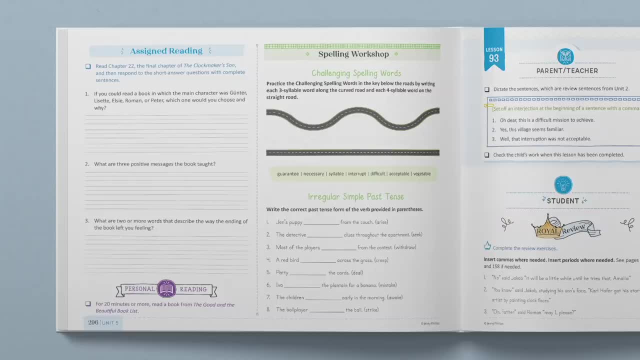 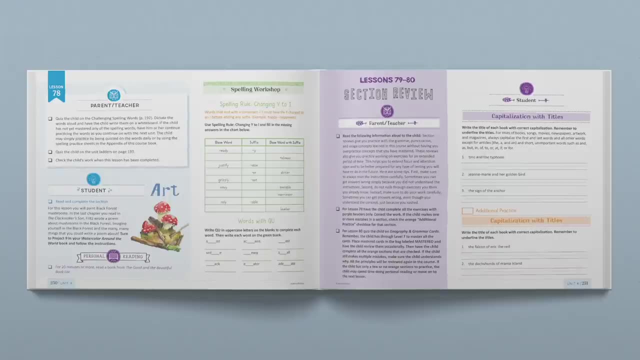 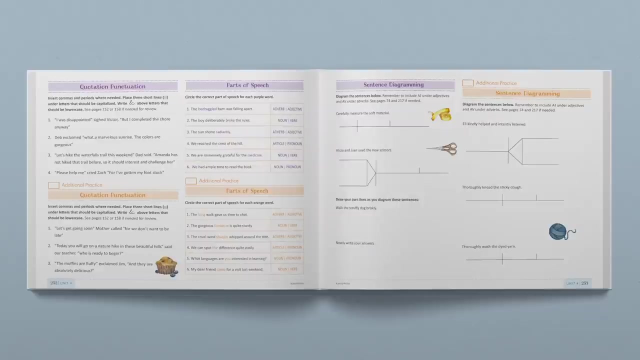 The student section contains grammar and assigned reading in the book The Clockmaker's Son, followed by reading comprehension exercises and then the child completes a spelling workshop. There are six units and each one ends with an assessment so you can check progress the child is making. The assessment includes extra practice for any principle the child does. 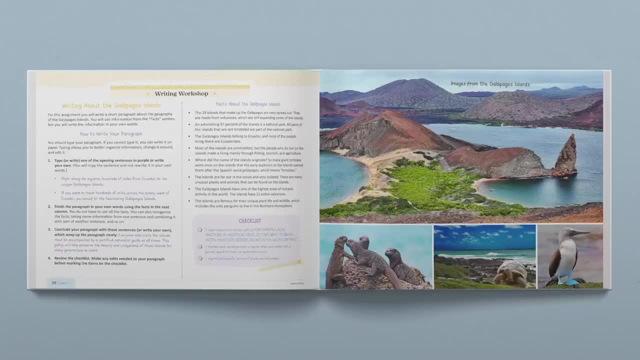 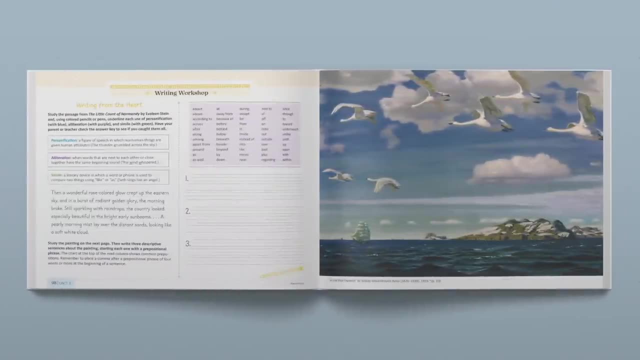 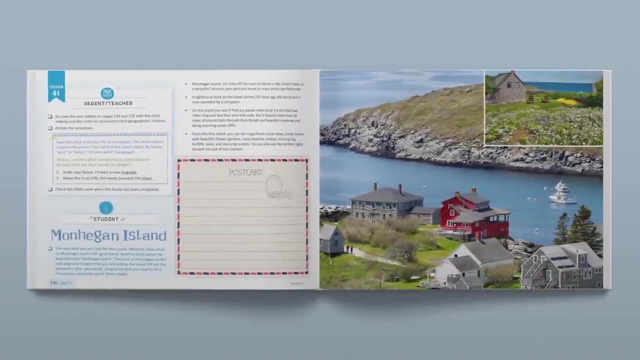 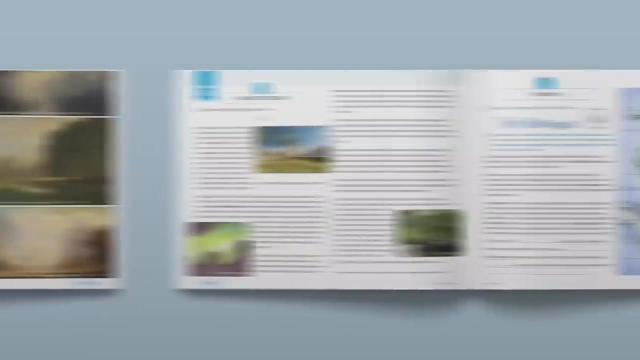 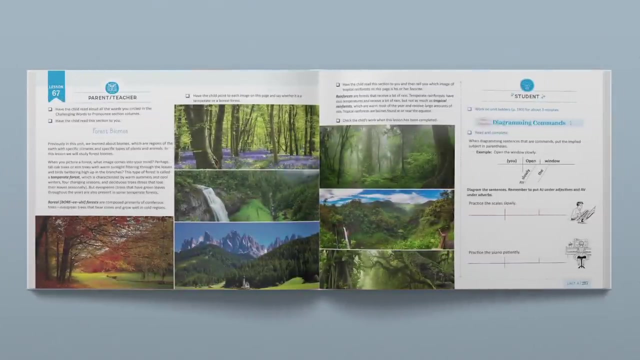 not pass. I'll end the video with a look at some other pages in the course book. Thank you for watching and don't forget to like the video. Thanks for watching.